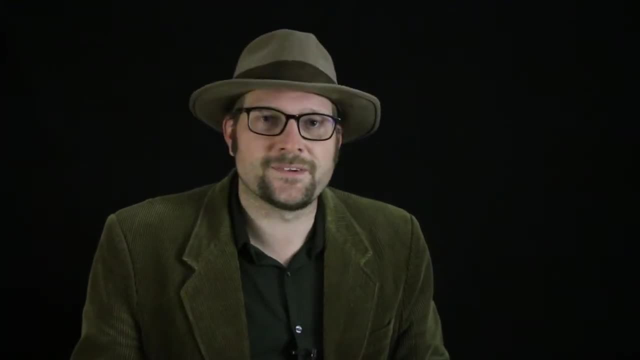 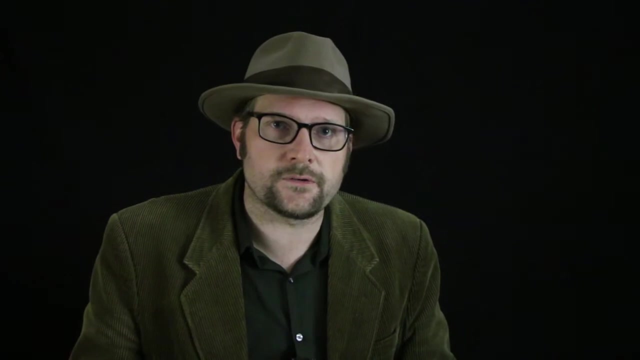 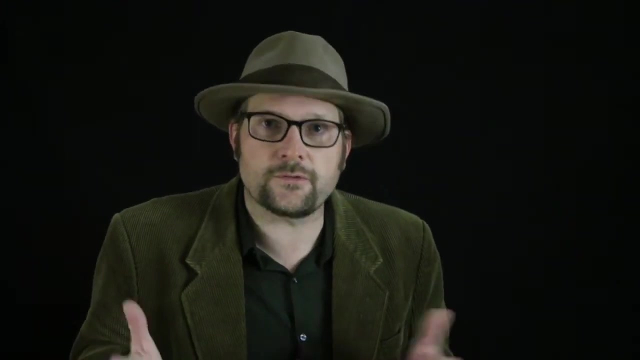 Welcome to Utah State University's Vertebrate Paleontology course. My name is Benjamin Burger and in this video we will interpret some of the unusual features of fossil birds discovered in the rock record of the Cenozoic and what some of these features reveal about the success of birds. over the last 66 million years. Modern birds quickly diversified during the early Cenozoic, although their origins are still masked behind a fossil record that does not reveal the earliest occurrences, until the Middle Eocene, when we begin to see the various groups of modern birds. 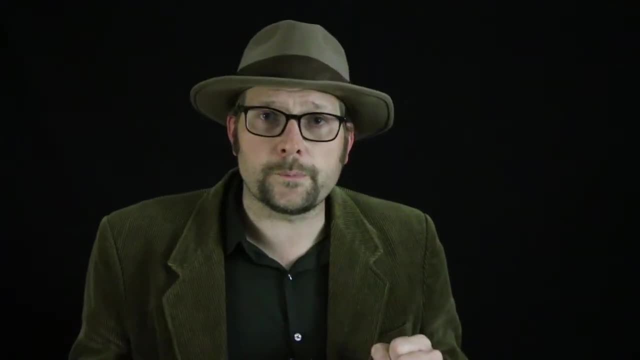 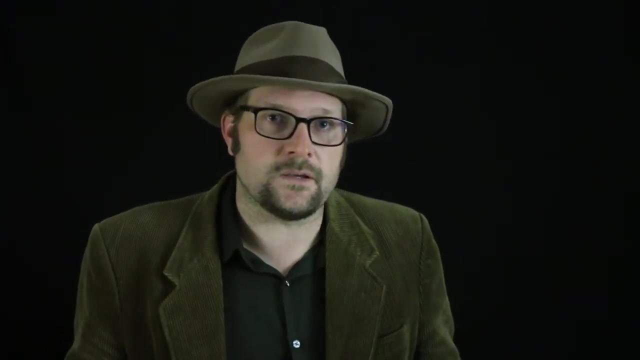 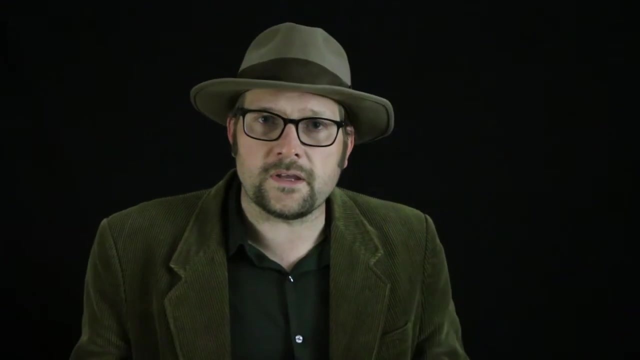 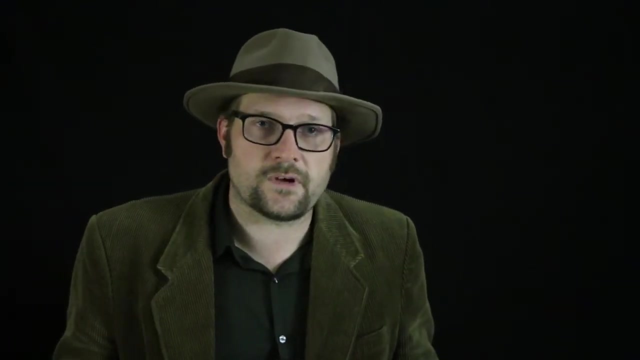 in the fossil record, There may have been multiple groups of modern birds that split apart during the late Cretaceous, with several groups surviving the K-T boundary extinction. So who were these earliest modern birds? There is good evidence both from molecular phylogenies of divergent times, as well as a limited fossil record during the late Cretaceous. 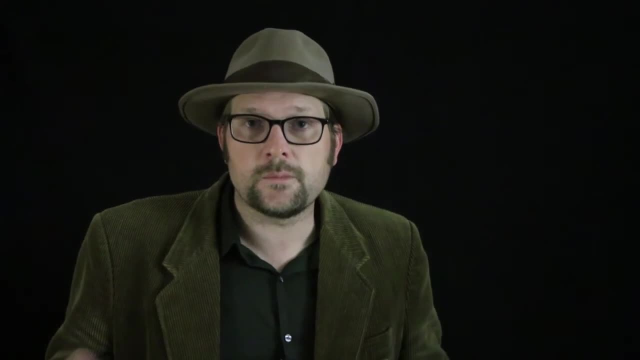 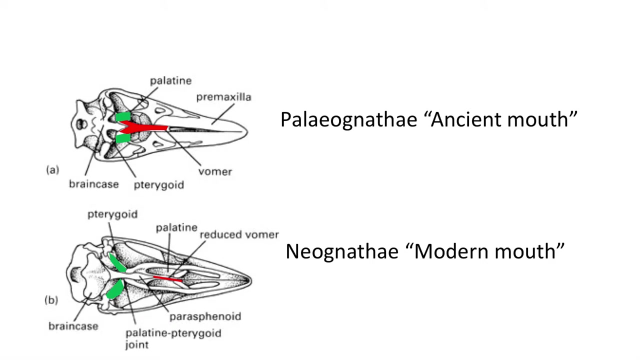 that two lineages of modern birds split before the mass extinction. These two groups of modern birds are called the Paleognathidae and the Neognathidae, which basically means the ancient mouth and the male and the female. The male is the most common species of birds and the female is 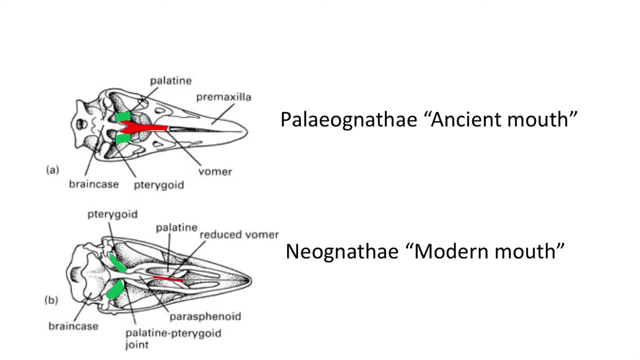 the most common species of birds. The male is the most common species of birds and the female is the most common species of birds. The male is seen in the males and the modern males, and both groups of birds live today. Next, the Paleognathidae birds are characterized by having a robust 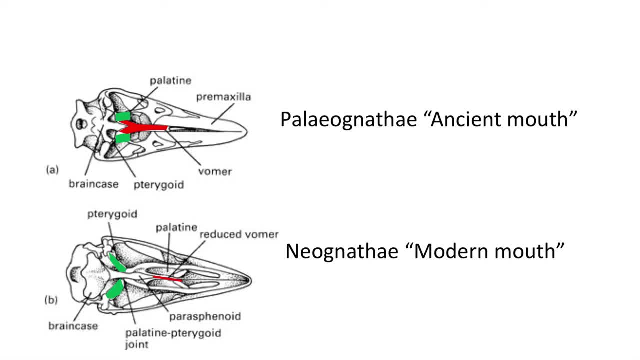 volmar that contacts the palatine bones near the back of the basal cranium In the Neognathidae. the volmar is highly reduced and the pterygoid bone is moved forward to contact the perisphenoid. The pterygoid bone is a very low-level bone that is usually played while. 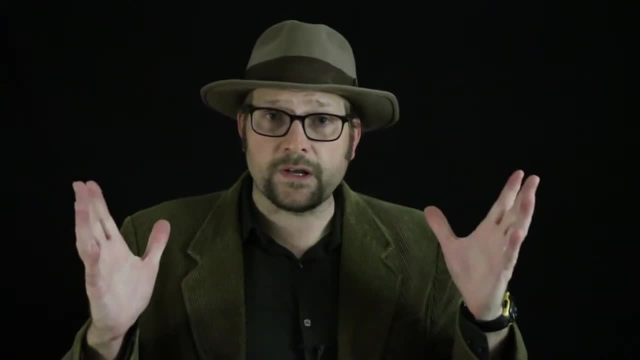 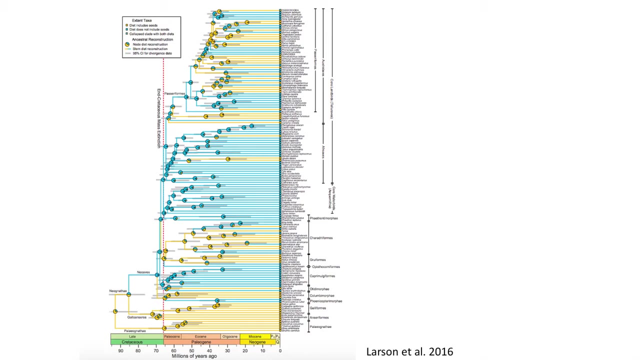 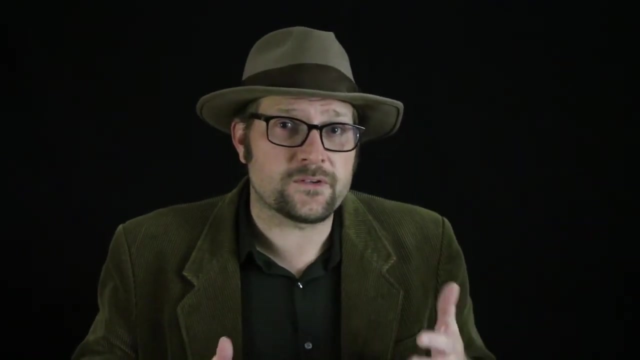 bone in the basal cranium. This division appears to have occurred prior to the end Cretaceous. although our fossil record of birds from the late Cretaceous is rather weak, A number of Paleognathid- igneognathid birds do appear during this time though. 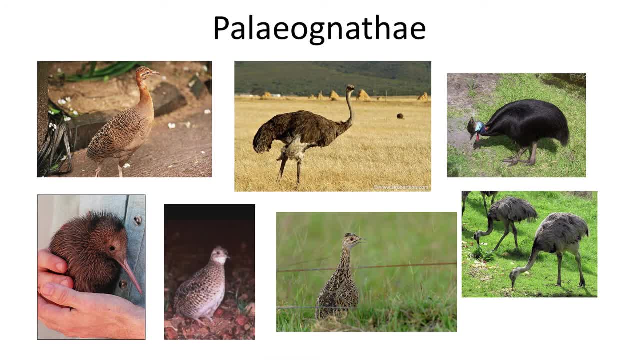 Today, the Paleognathid birds are represented by a diverse group of ground birds and some are flightless. They have a Gondwana land distribution found in South America, Africa, Australia, as well as islands in the Pacific and Indian Oceans. 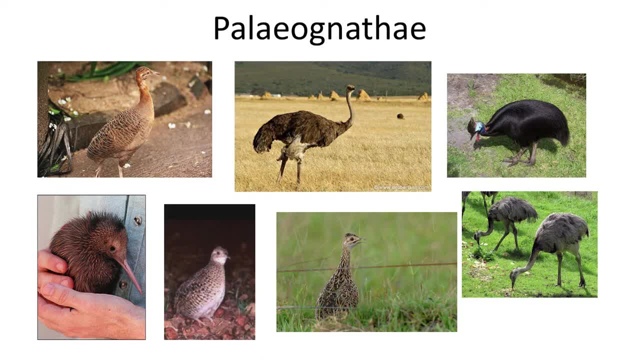 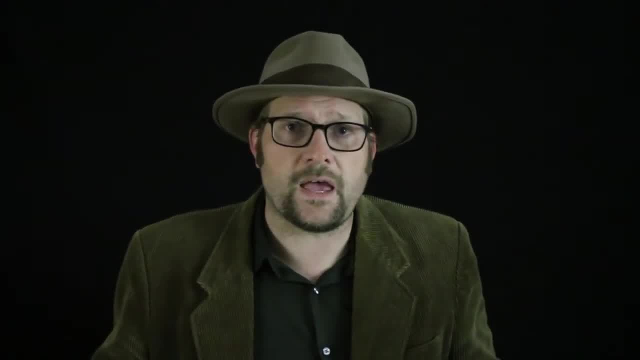 They include ostriches, kiwi birds and the titimu. While some Paleoornithologists have placed several Cretaceous birds into the Paleognathidae, such as Gobiopteryx, recent phylogenies tend to recognize most of these early Cretaceous. 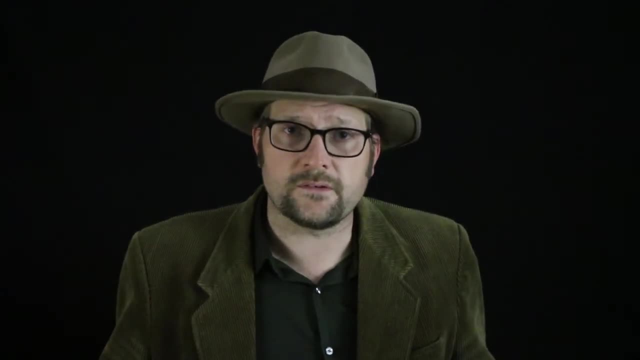 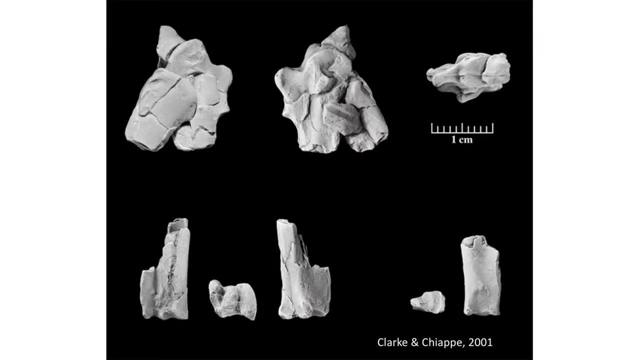 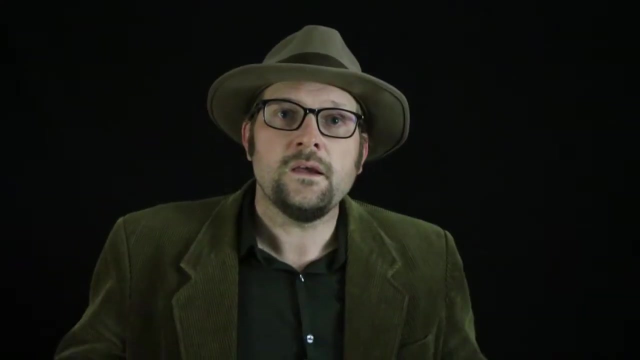 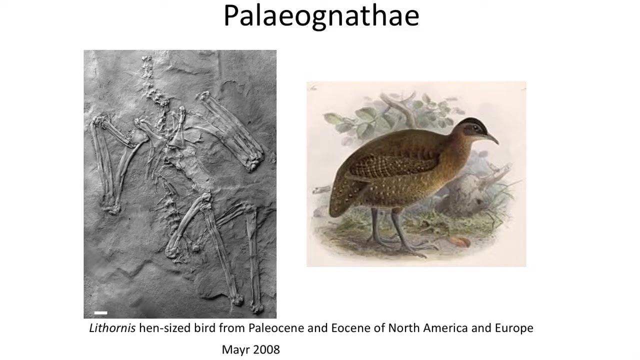 fossils as members of the Enantodon In the Paleocene and Eocene. a number of better preserved Paleognathid birds are known, including Hornis, which is a hen-sized bird from the Paleocene and Eocene of Europe and North America. 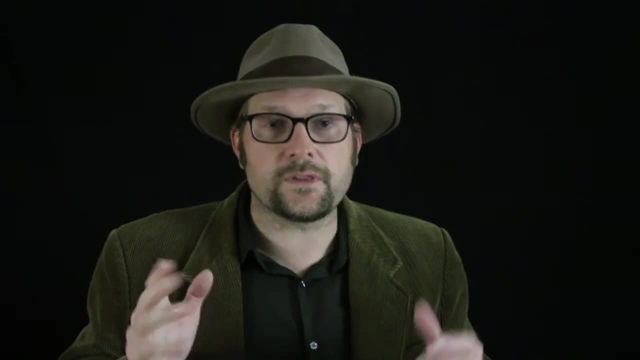 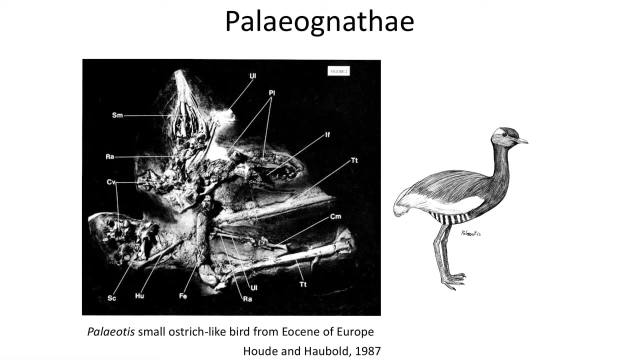 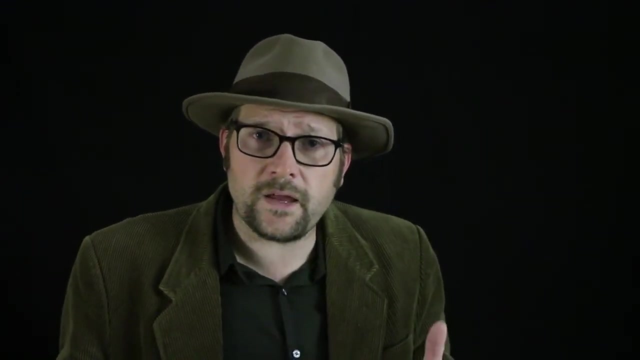 indicating that the group was more globally distributed during the early Cenozoic. Another early Paleognathid bird is Palaeotis, from the Eocene of Europe, which was a small ostrich-like bird, indicating that several of these groups became flightless during the. 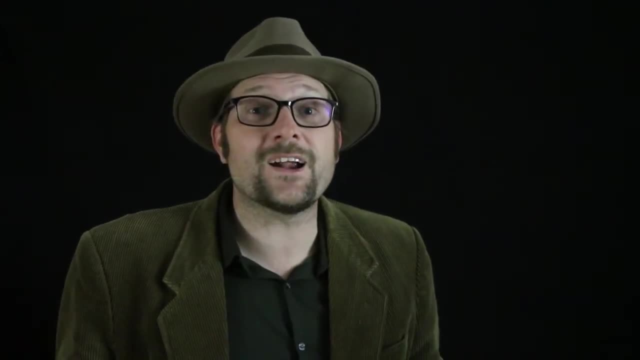 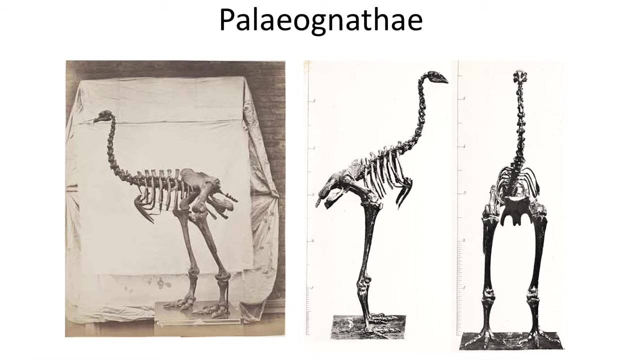 early Cenozoic And some became very flightless. The largest of the Palaeognathid birds are the giant Moa of New Zealand, which sadly only went extinct just 500 years ago. The islands of New Zealand lacked any mammalian predators and these birds were able to dominate. 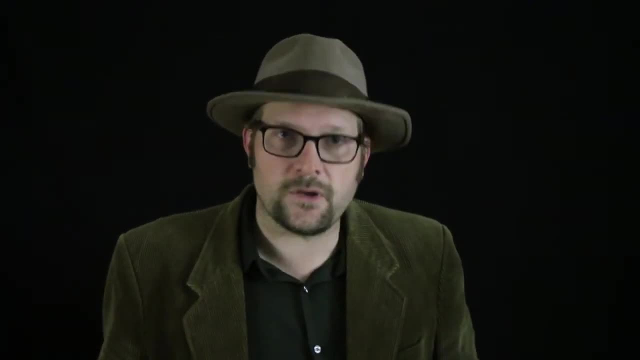 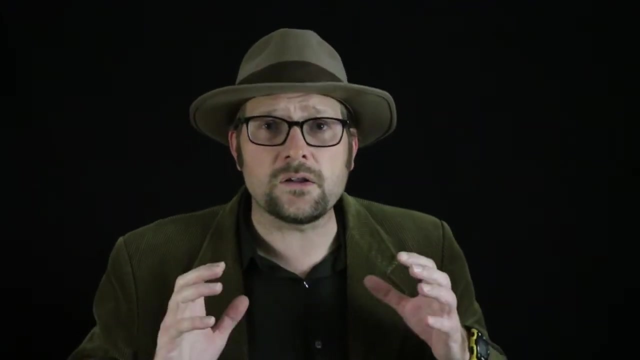 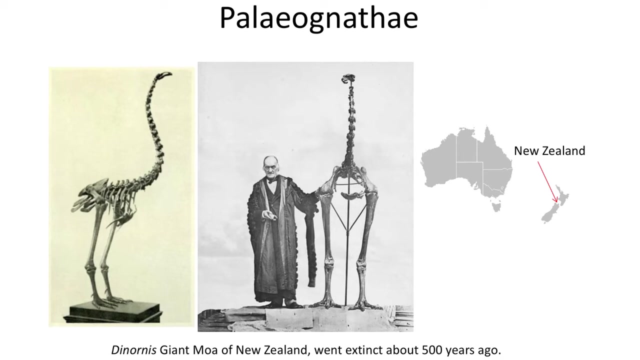 the ancient ecosystem until the arrival of humans. The birds stood almost 3.5 meters tall and weighed 250 pounds. The discovery of the giant Moa, or Deina Hornis, is an interesting story. In 1839, Richard Owen had purchased a bone that had been found in the mud of one of the 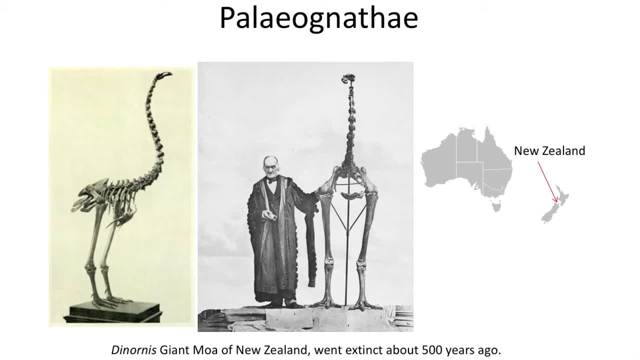 bays in New Zealand and he found that it closely resembled an ostrich but was much bigger. He hastily published a paper describing an extinct large bird from New Zealand, but few people believed him. Then in 1843, someone sent a bunch of bones to William Buckland at Oxford and he recognized 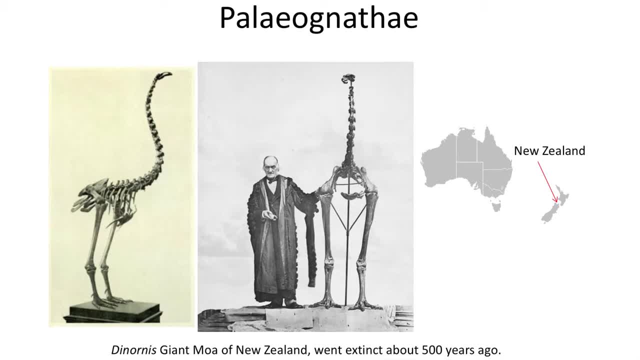 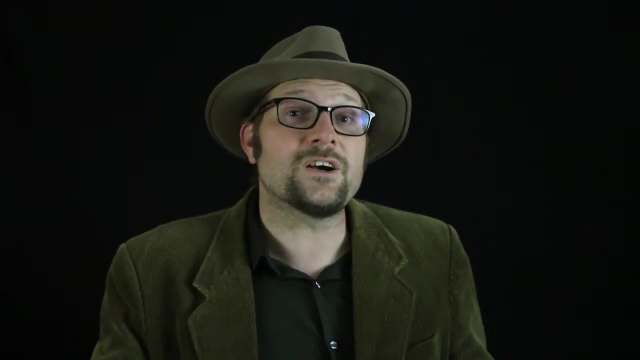 them as Owen's giant bird and he sent them to Richard Owen to describe The following paper describing the reassembled skeleton. and it was a sensation, as Richard Owen had previously predicted a giant extinct bird in New Zealand. New Zealand is not the only island nation with large extinct birds. 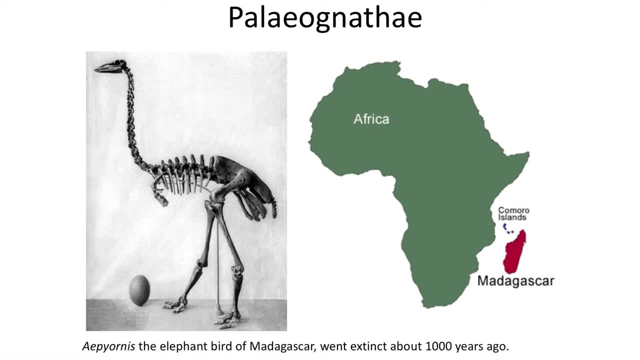 The island of Madagascar had a large extinct bird called the Elephant Bird or Egypta Hornis, which is closely related to Deina Hornis. It went extinct about 1,000 years ago, also succumbing to extinction after the arrival of humans to the island. 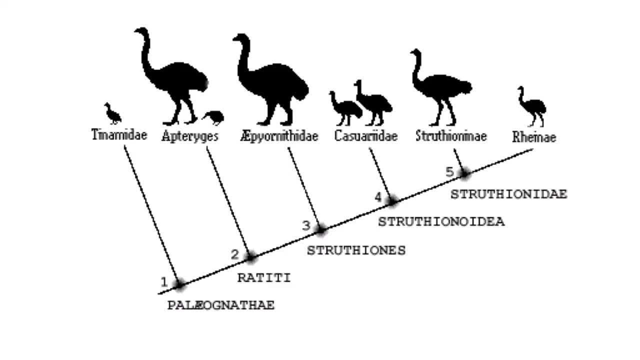 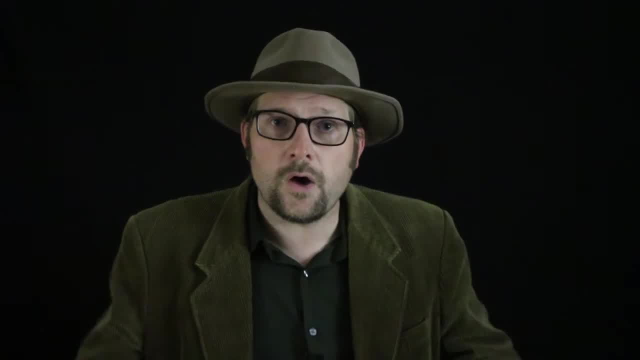 The Palaeognathid birds are composed of both flightless and flying birds, which were able to colonize these islands where they lost the ability to fly, Although ostriches are members of this group and they live in Africa, where they are fast. running birds and live on the African savannah. The next group of birds that arose during the late Cretaceous are the Neognathidae, which includes over 140 families and over 9,000 species. Most of the earliest members of the Neognathidae clade appeared during the Middle Eocene, with 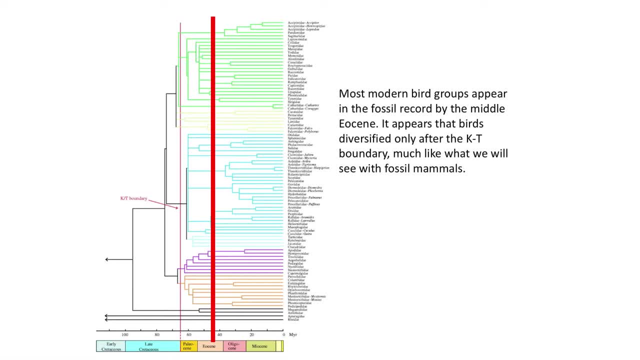 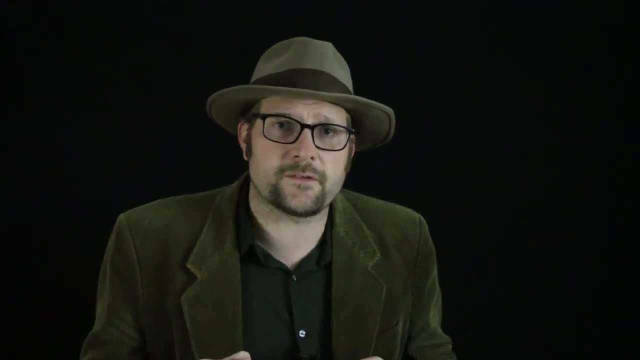 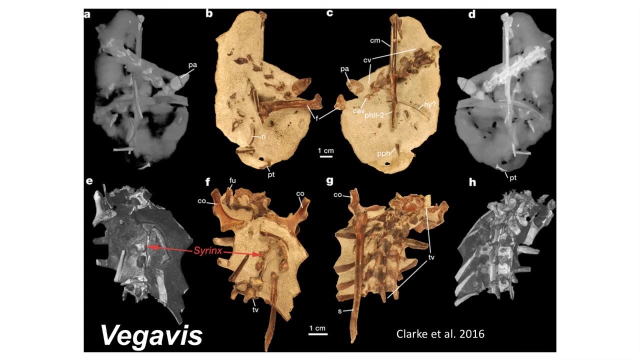 most groups differentiated by 50 million years ago. Two of the earliest Neognathidae birds are some unusual fossil discoveries made in the late Cretaceous of Antarctica. Vegeavis was described recently and it features a modern Syneryx, which is a vocal box that 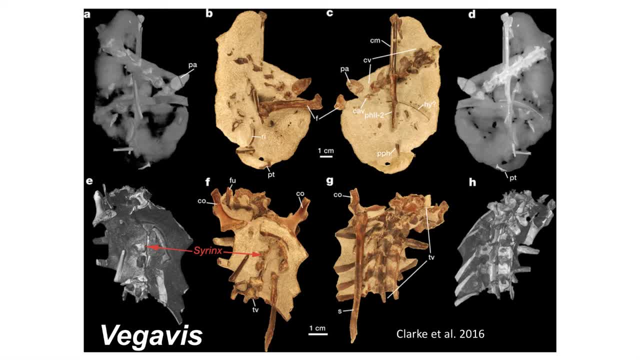 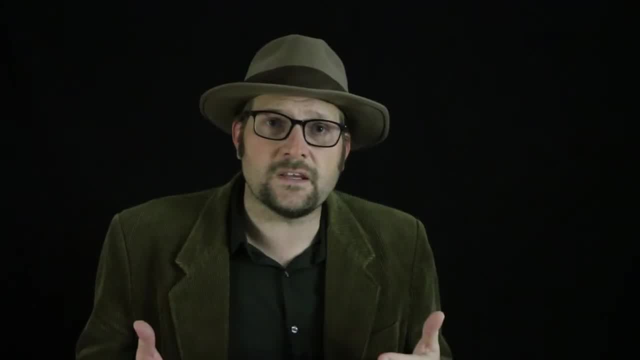 is located at the bottom of the sea, At the split in the trachea between the two lungs, And it is used by modern birds in making their vocal calls. Vegeavis is a duck-like bird which is in close relationship to another fossil from. 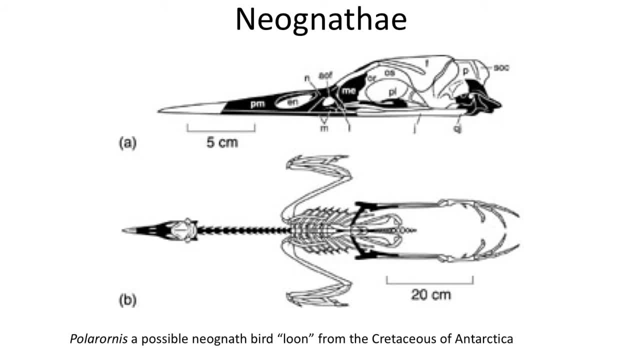 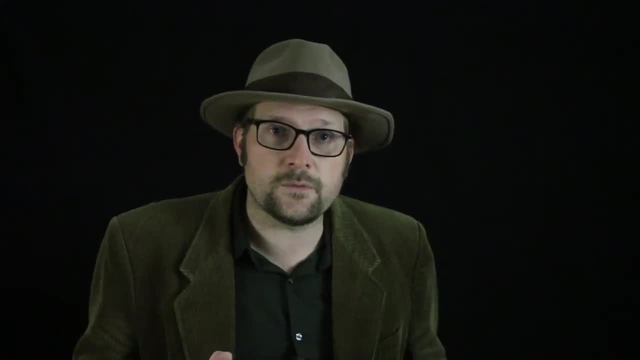 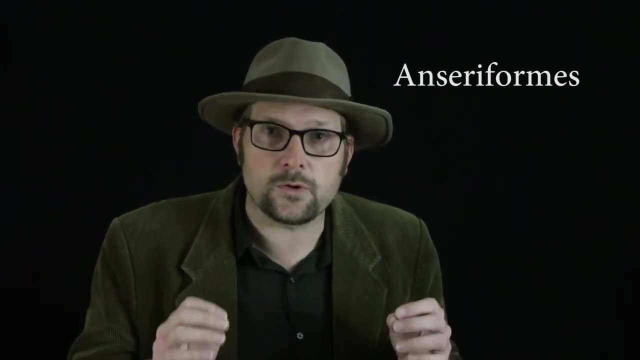 the late Cretaceous of Antarctica, Polioornis. Both of these late Cretaceous birds are considered members of the Neognathidae and are believed to be in the modern group of birds called the Anansiformes. They include ducks, geese and loons and are closely related to the Galeiformes, which 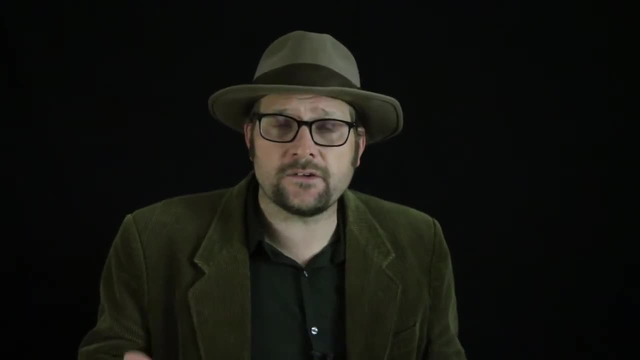 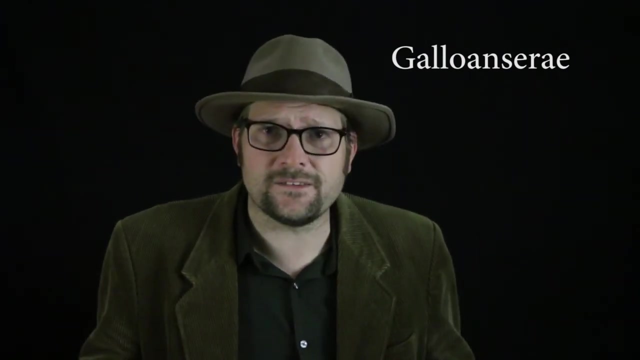 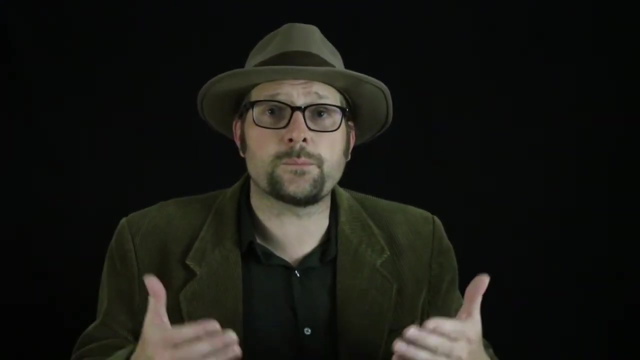 include chickens. This clade is called the Galeansirae in our textbook. The fossil record of the Galeansirae- the ducks and chickens- are remarkably good during the Eocene. One of the more common fossils in this group is Prisporornis, where a number of skeletons 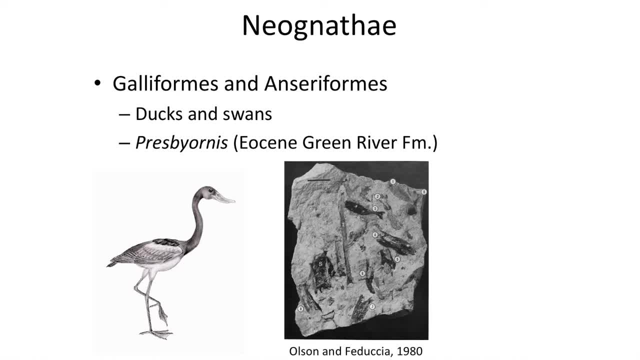 have been found in the Eocene lake system. Prisporornis is one of the largest species of geocene in North America and it has a fossil record that extends all the way back to the Paleocene. Prisporornis had a duck-like bill but featured long legs like a crane or stork. 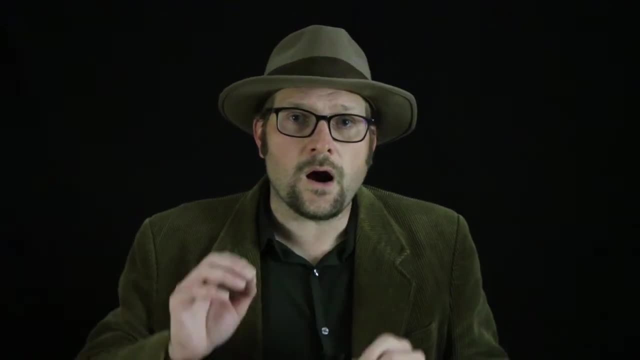 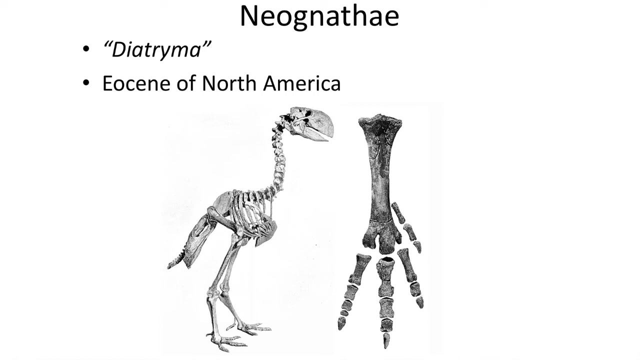 One of the most unusual of the Galeansirae are the giant, flightless Neognathidae birds that evolved in the late and Eocene in Europe and North America. The North American genus is called Diatrymae. 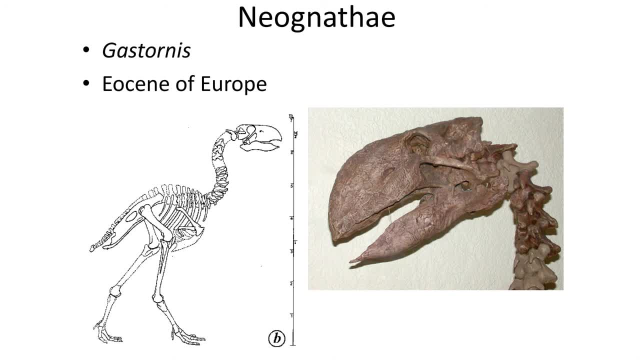 European genus is called Gastroornis, and some researchers have synonymized them into just Gastroornis. This was a giant bird that measured over 2 meters high. One of the best specimens was found in the Wilwood Formation in Wyoming, and they are. 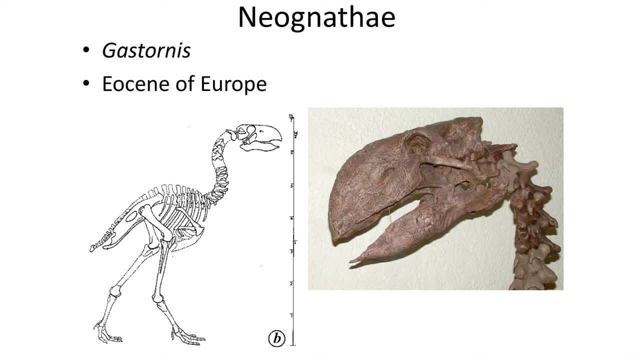 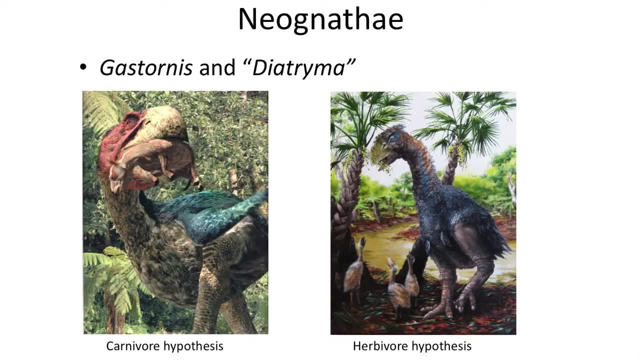 sporadically found in the Eocene of both continents. There has been considerable debate over what Gastroornis ate. One theory holds that it was a carnivore which used its strong beak to hunt small mammals. The other is that they were herbivores using their strong beak to crack large nuts. 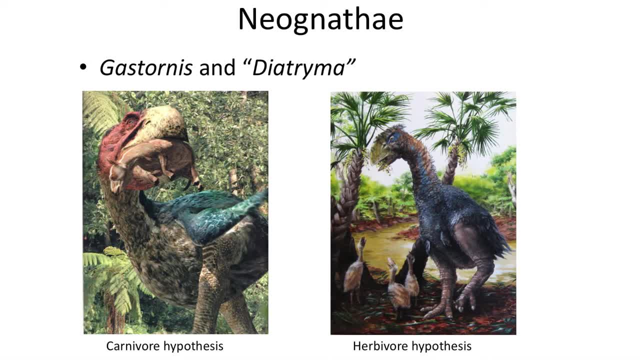 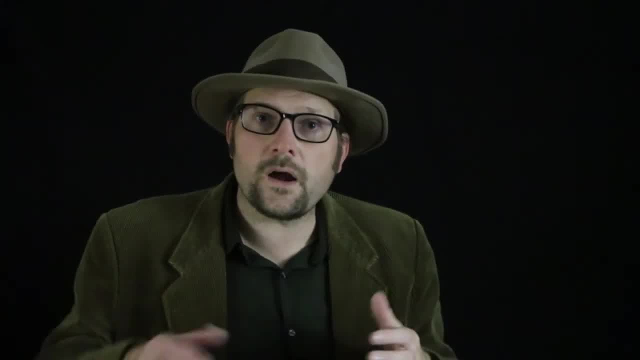 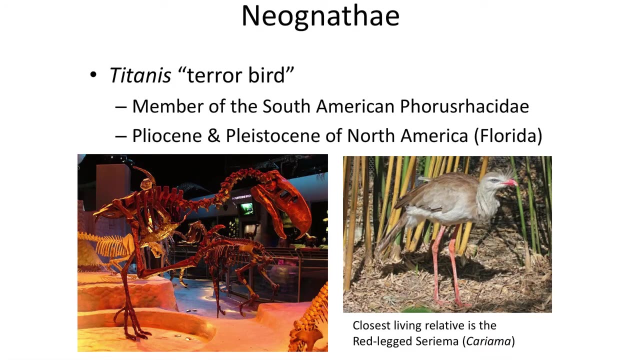 One thing supporting the herbivore diet is the fact that it lacks a hooked beak like those found in owls and hawks. Another unrelated giant bird that evolved in the Cenozoic were the tare birds of South America. These large carnivorous birds arose during the Neogene and migrated into North America. 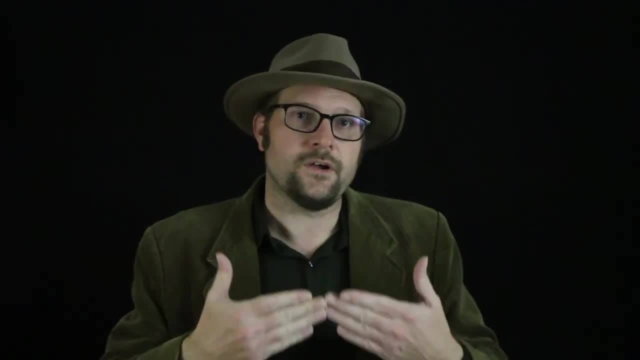 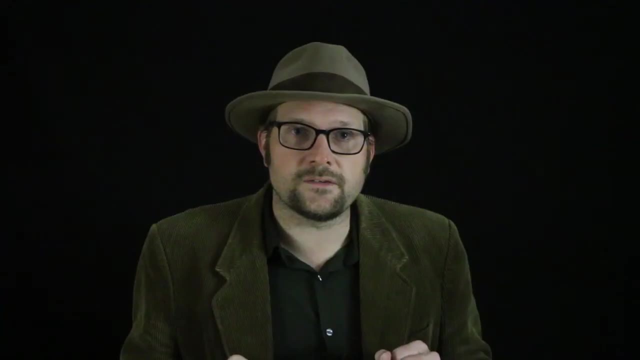 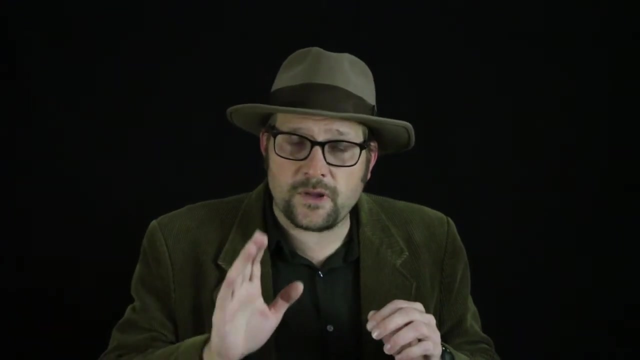 after the two continents came in contact with each other during the Pliocene. Their closest living relative is the red-legged Ceramera and featured hooked bills which are unlike Gastroornis Titanus, measured up to 2.5 meters tall and is found in the Pliocene. 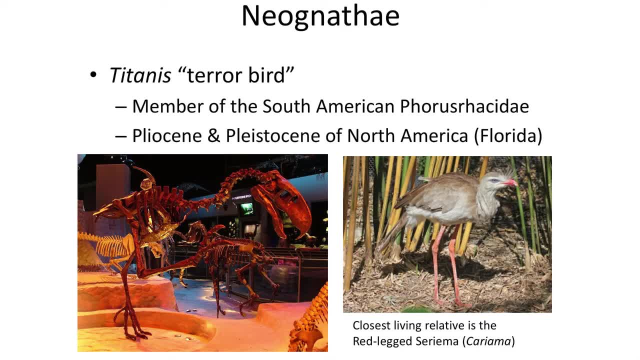 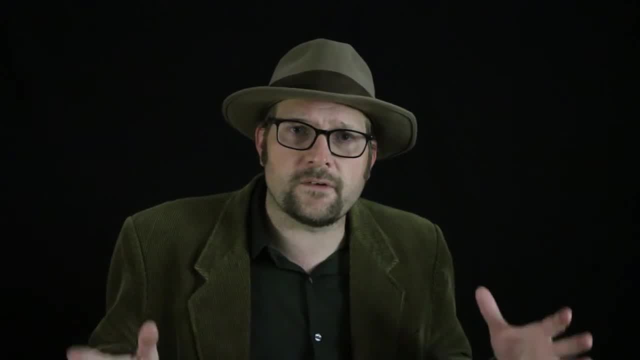 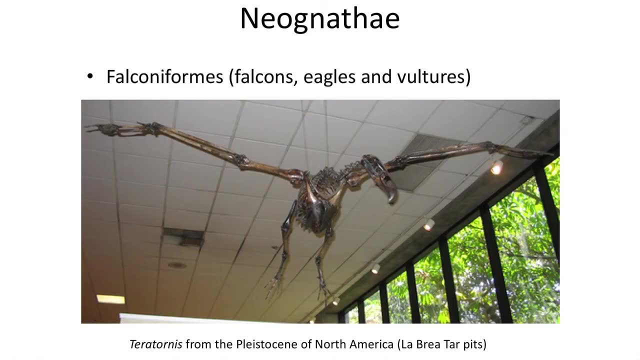 The interrelationships of the Neonathidae is fairly complex, although most groups have a fossil record that dates back to the Middle Eocene. This includes forms like Falchiformes, which have a fossil record back to the Late Palaeocene. 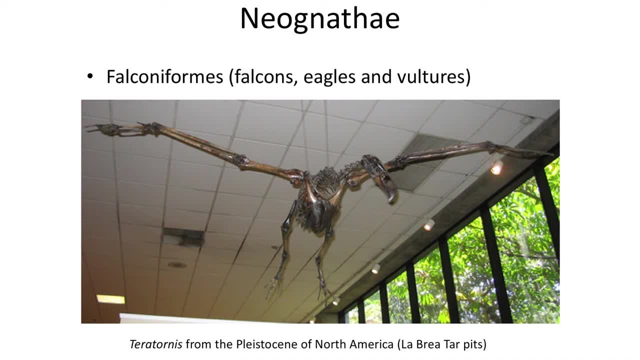 One of the richest fossil bird sites is the La Brea Tar Pits in Los Angeles, in which thousands of fossils of the Neonathidae are found. This late Pleistocene site was a natural trap for these vulture-like birds, which became 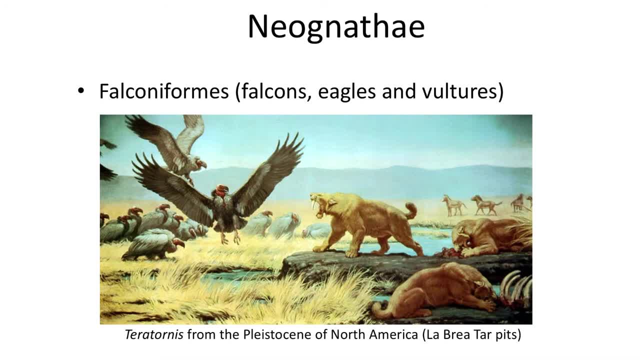 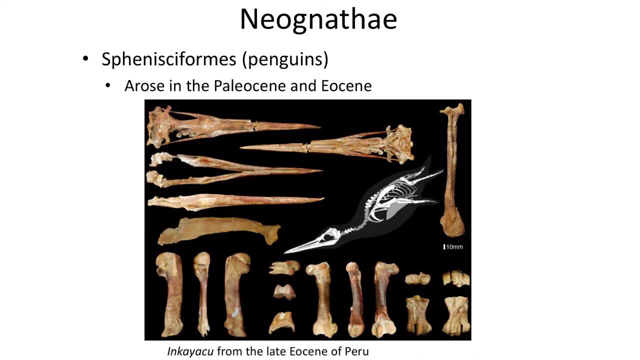 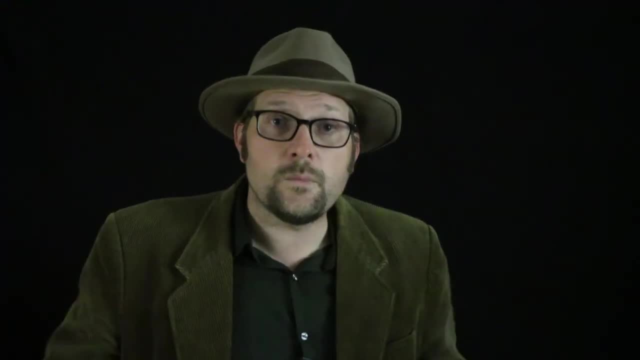 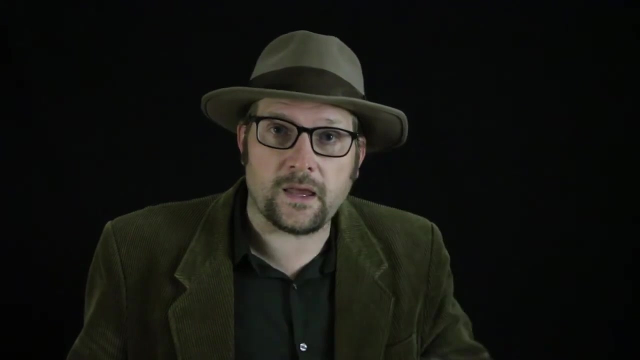 stuck in the tar as they tried to feed on trapped mammals. Another group of birds with a fantastic fossil record are penguins, which first appear in the Late Palaeocene and were well represented by the Middle Eocene. Penguins are found in coastal depositional environments in South America and Antarctica. 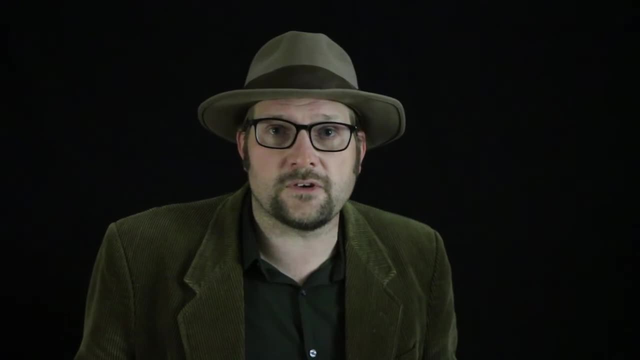 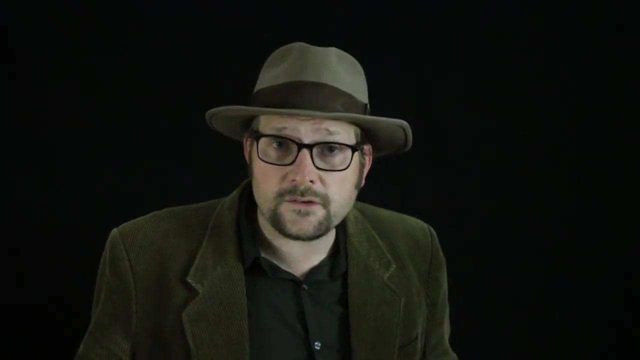 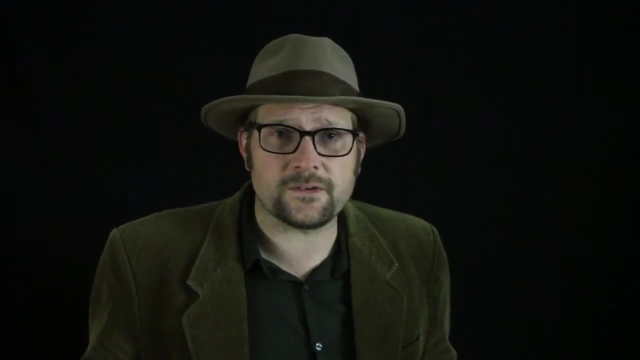 indicating that penguins arose before the ice ages that covered Antarctica in ice sheets. Penguins live in the Southern Hemisphere, where their fossil record is also limited to Some Eocene and Oligocene fossil penguins got rather large, about 2 meters in height. 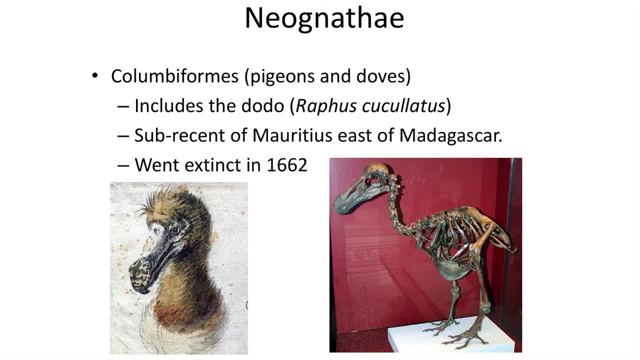 One group that I'll pause at are the Cubliaformes. They are a group that contains the Eocene and Oligocene fossil penguins. They are a group that contains the Eocene and Oligocene fossil penguins. They are a group that contains the Eocene and Oligocene fossil penguins. 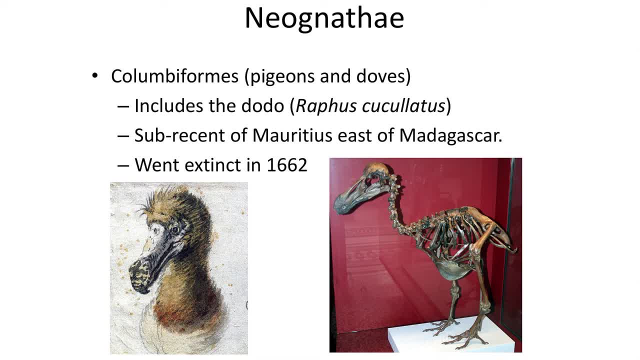 The Cubliaformes are the extinct Dodo bird, which lived up to 1662 on the Mauritius Islands, east of Madagascar. The Dodo bird has come to symbolize extinction like no other organism, as the extinction of the bird was well documented by sailors and explorers to the island. 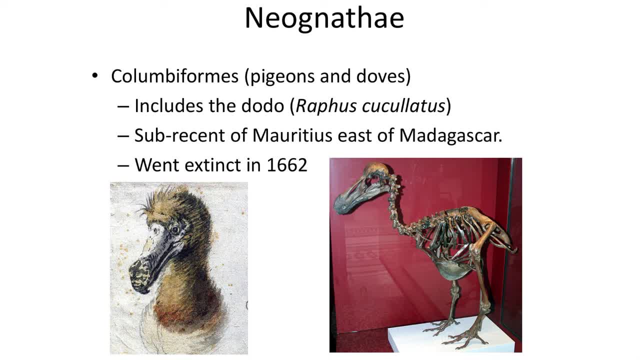 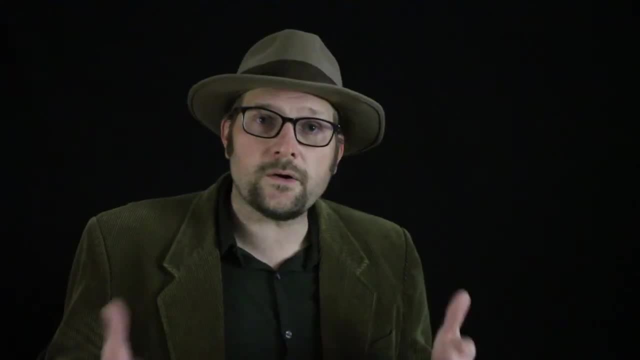 Human hunting, as well as the introduction of domestic animals to the island, doomed the little bird, which was flightless. This sketch is the only image we have of a living Dodo bird, and only a handful of skeletons have made it into museums. 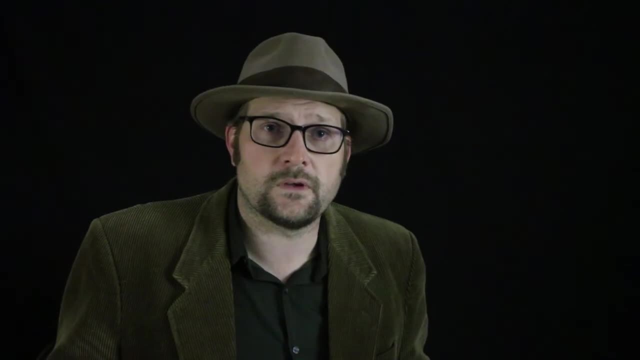 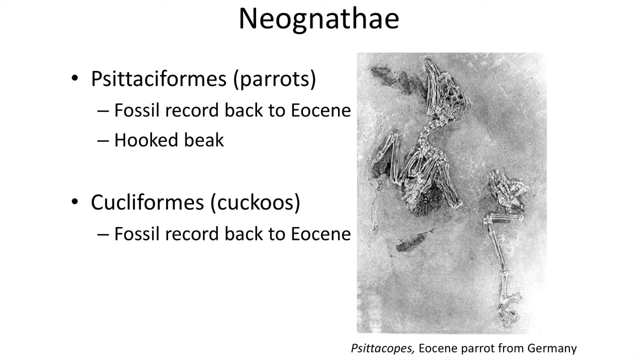 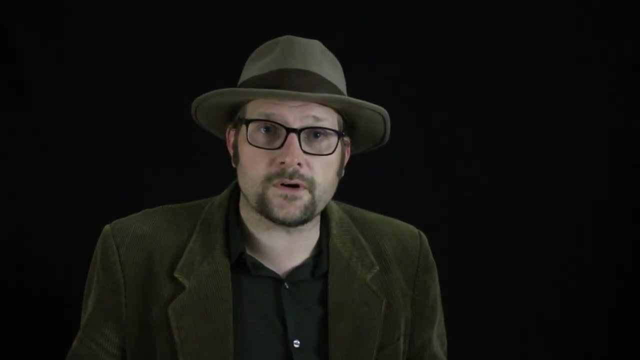 Parrots are another unique group of highly intelligent birds and they have a fossil record dating back to the Eocene, with several forms known from Germany. They are closely related to the Cuckoos, The last group of Neonathid birds to arise, are one of the most diverse of the living 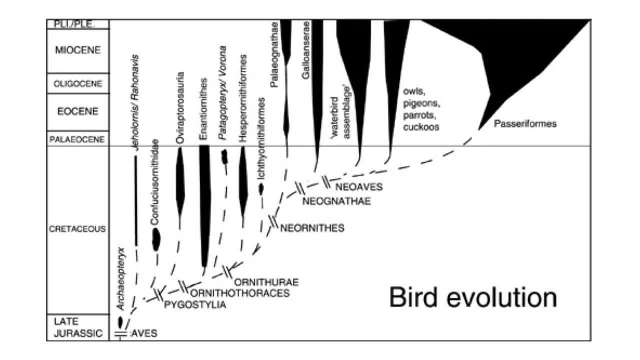 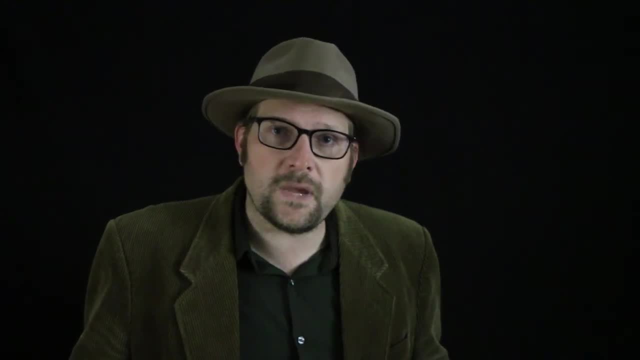 modern birds, the Passiformes, which include songbirds and perching birds. The group arose rather recently in the Miocene. some ornithologists believe they rose even earlier but quickly became very diverse during the Miocene to make it into the fossil record.